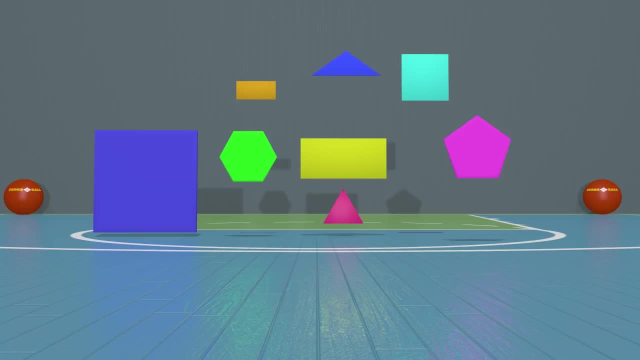 these can help us know which shape is which. So let's take a closer look. Here we have a triangle, But what makes this shape a triangle? For a shape to be a triangle, it must have three sides and three angles. This shape has one, two, three sides. Okay, it has three sides, but does it have three? 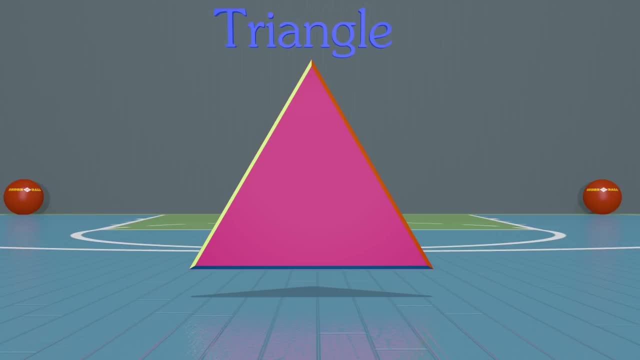 angles. Well, the angle is where two straight sides join together. Sometimes the angles are called corners. We can see that this triangle has one, two, three angles. So this shape is a triangle because it has three sides and three angles. Now, how about this shape? This? 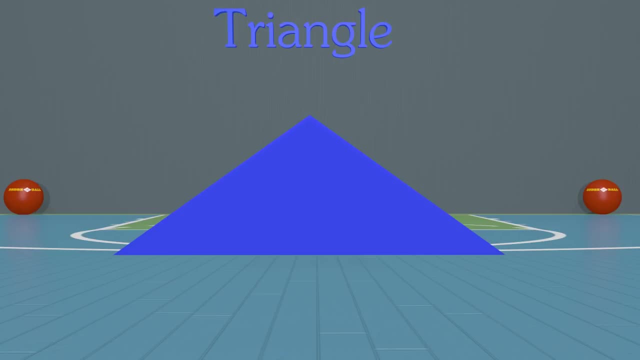 looks a lot like the other shape, but it's more squished. Is this still a triangle? Well, let's count the sides and angles and see what it is. Okay, we have one, two, three sides and one, two, three angles, Three sides and three angles. That means that it is a triangle. 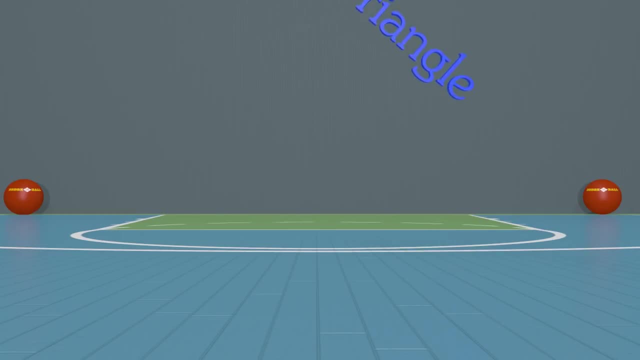 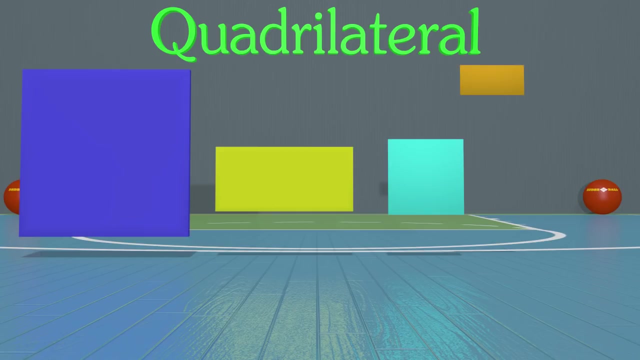 Great job, guys. Okay, let's look at some more shapes. Now we're going to look at quadrilaterals. A quadrilateral is any shape that has four sides and four angles. Many shapes can fit the attributes of a quadrilateral. Here are: 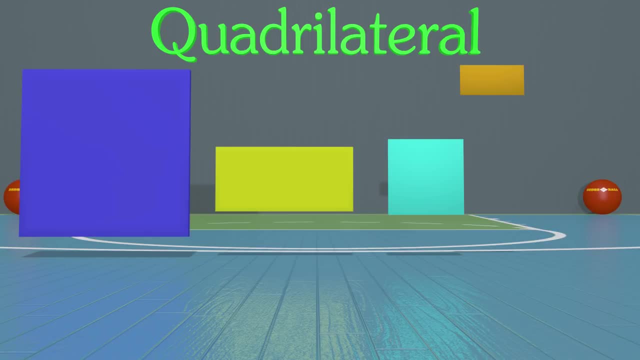 a couple quadrilaterals. Let's learn the names of these shapes. The first shape is called a square. The next shape is called a rectangle. What is this next shape? Great job, This is a square like the other one. What is this last shape called? You got it. This is another rectangle. 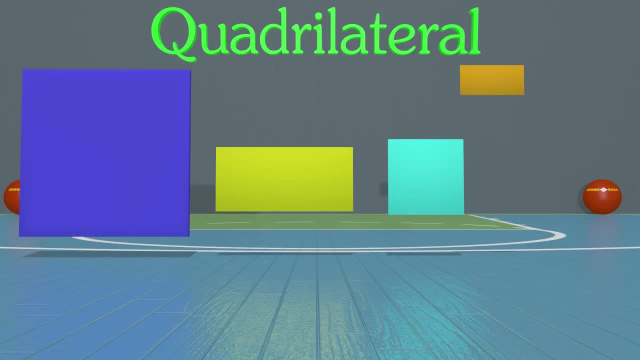 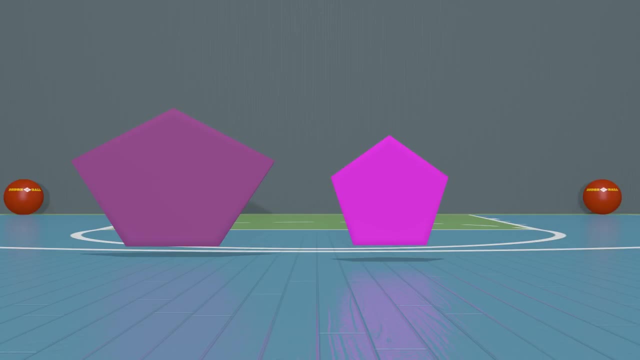 All of these shapes are quadrilaterals because they have four sides and four angles. Wow, These shapes have a lot of sides and angles. Let's count how many sides are on this shape. There's one, two, three, four, five. How many angles do you see? Five, It has five.